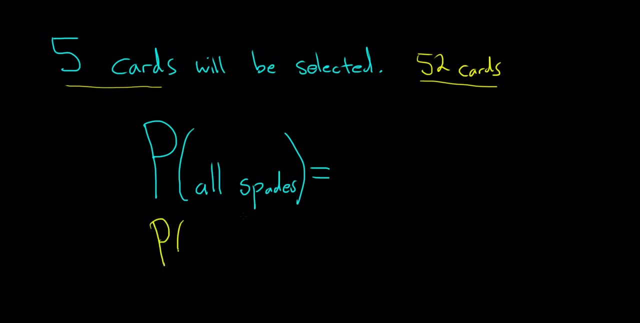 this is as follows. So if they're all spades, that means that the first one is a spade and the second one is also a spade, and the third is a spade, and the fourth and the fifth. So the first is a spade, the second is a spade, the third is a spade, the fourth is a spade. 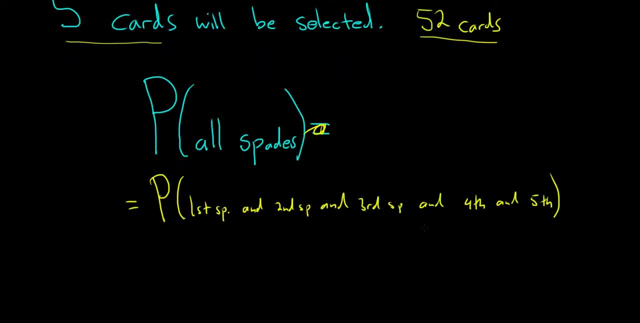 and the fifth is a spade. And the key to at least mentally figuring this out is to realize that the word and is there, So you don't have to think about it as a whole. You don't have to think about it as a whole. 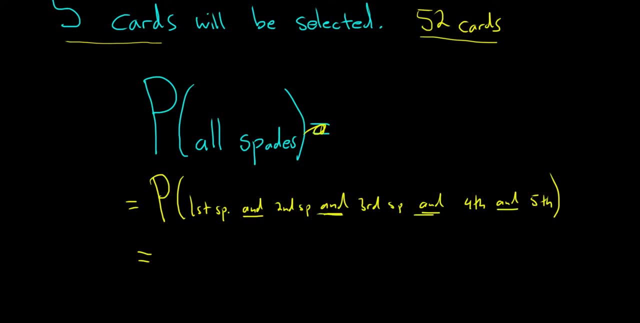 You don't have to write it down, but as long as you know the word and is there that tells you to multiply. So now we just do each individual probability and we multiply. So first we want the probability of picking a spade card. Well, there are 13 ways to pick a spade card and there 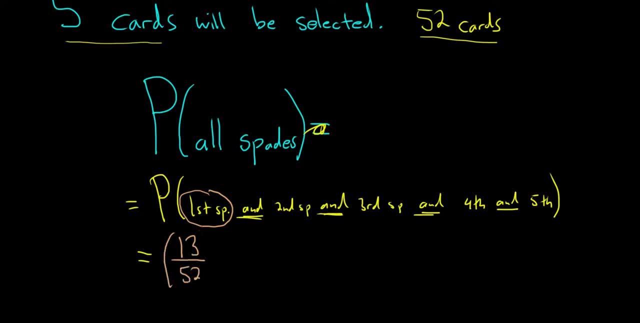 are 52 ways to pick a card. So the probability of picking a spade card is the number of ways to pick a spade card divided by the number of ways to pick a card, And the and tells you to multiply. So you want the second card to be a spade card. Well, you've taken a spade card out, so now there are only 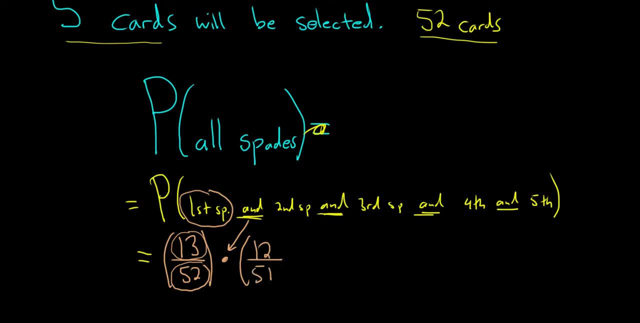 12 ways to pick a spade card, and then there are 51 ways to pick a card. And now the third one- now there's only 11 spade cards and 50 cards- And the fourth one, so 10 over 49, and the very last one. 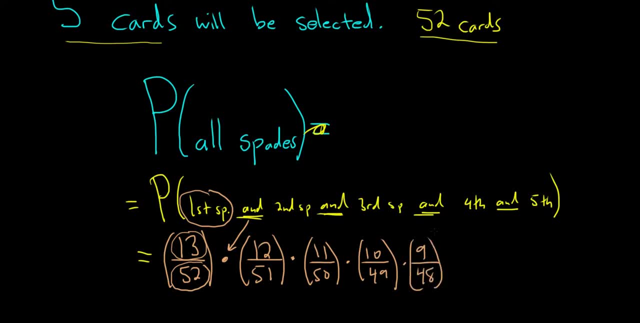 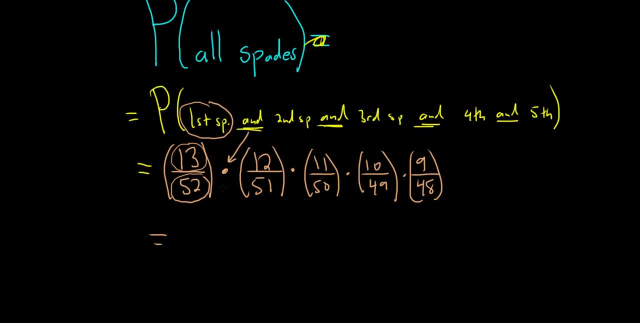 would be 9 over 48.. So now we just have to put this huge fraction in our calculators. So I haven't done this problem yet, so I'm going to type it into my calculator, And if you're typing it into your calculator also during this moment, it's really important. 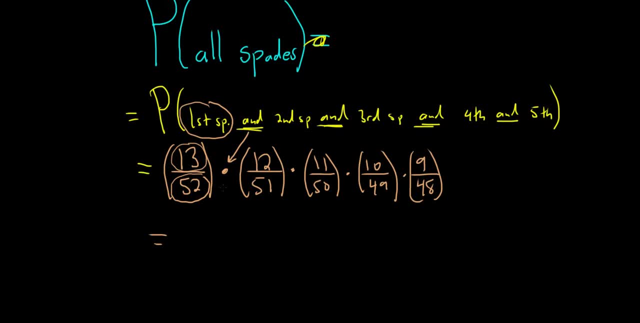 to include the parentheses, as I have on the screen. Without those parentheses, on many calculators you won't get the correct answer. So here we go. I'm about to hit enter. Just double checking that I've typed it in. Yes, that's what I thought we were going to get. So my calculator says: